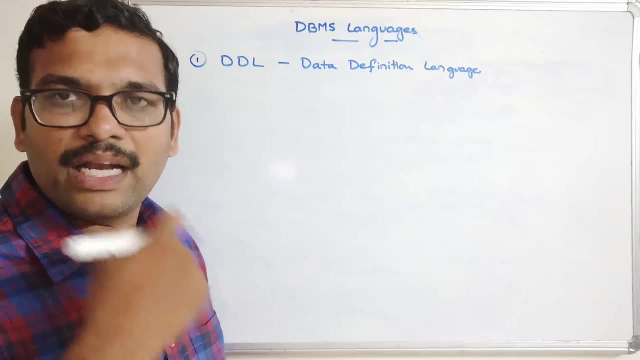 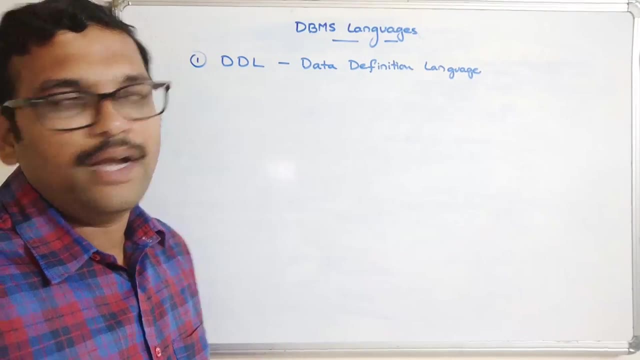 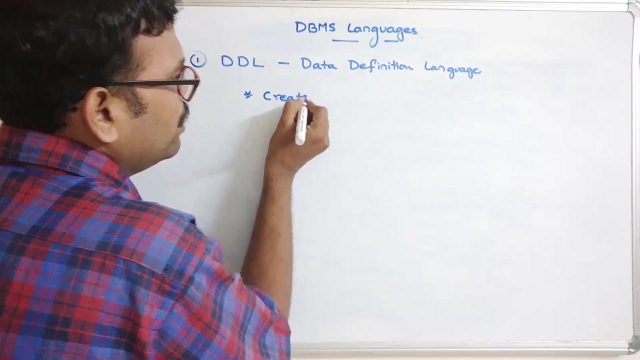 structure of database, not the data of database. So the database will be having some data, but these DDL commands will work on the structure. That means the skeleton of database. So the commands comes under this. DDL are the first one, create. So this command is used to create. 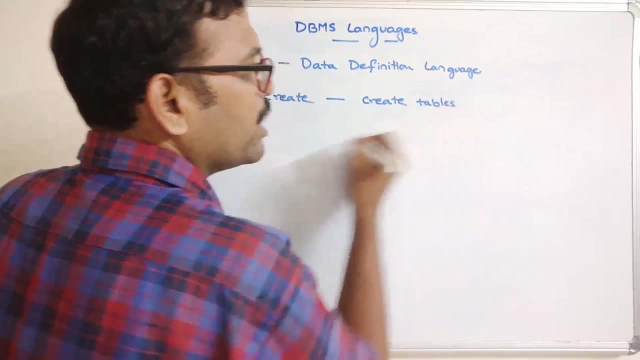 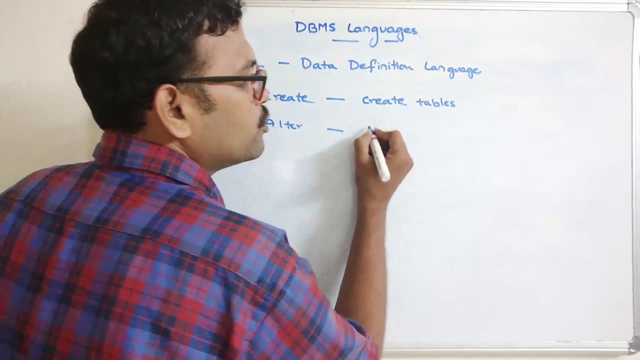 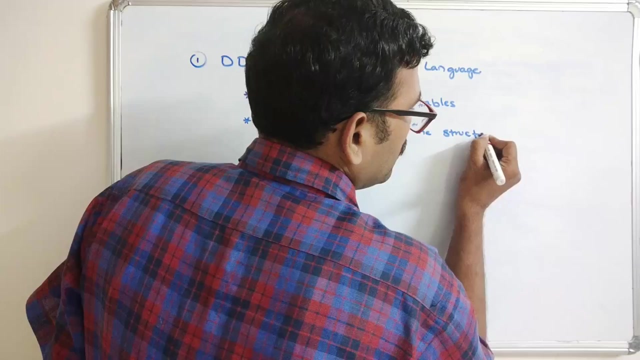 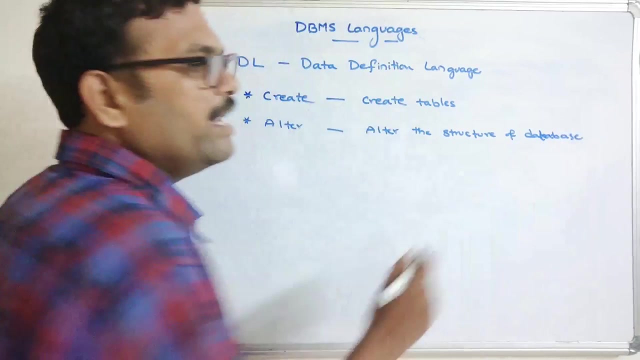 a database, I mean the tables or objects. Create a tables or objects And the second one alter. So this command is used to alter the structure of database. So altering the structure means adding some more attributes, removing some attributes, whatever it may be, that comes under this alter. 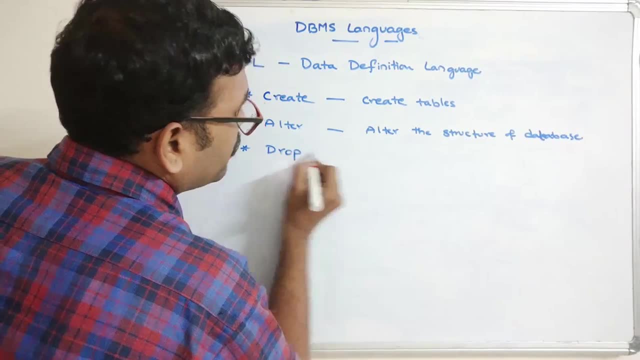 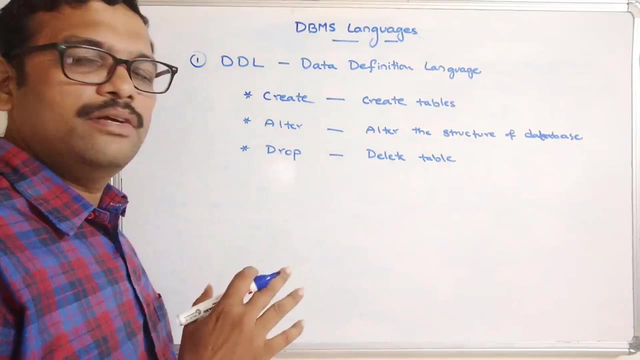 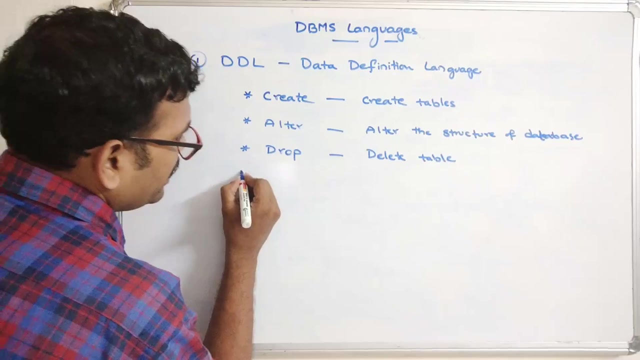 Next one: drop, So this is used to delete the table. Entire table: Okay, not the data. So all these commands will be working on the structure of database schema- Okay, not the data in the database. and the next one: truncate. So this truncate is used to remove. 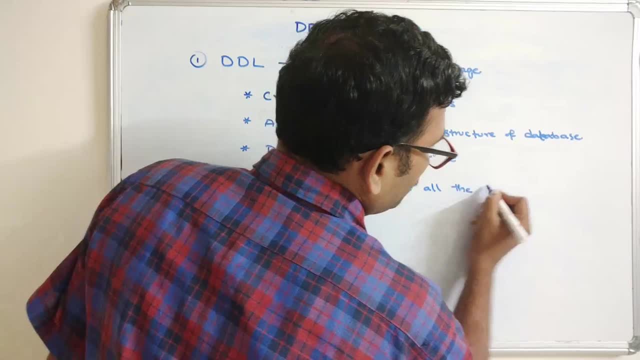 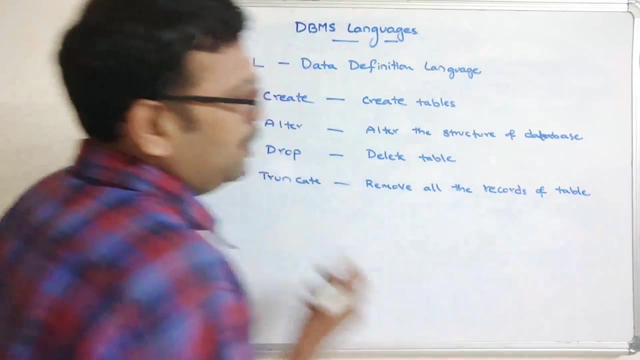 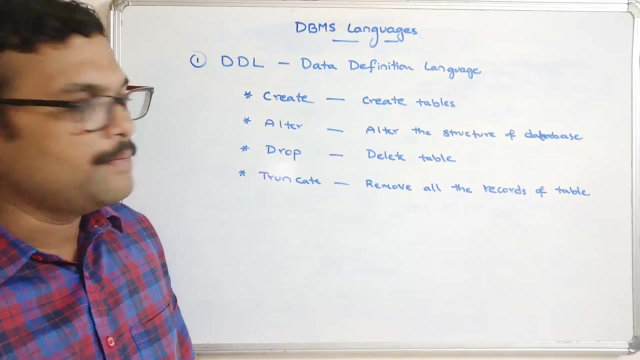 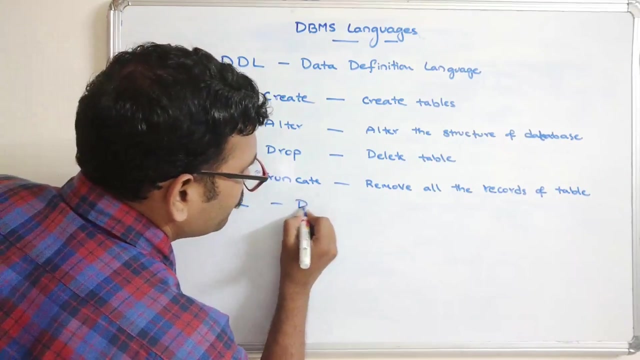 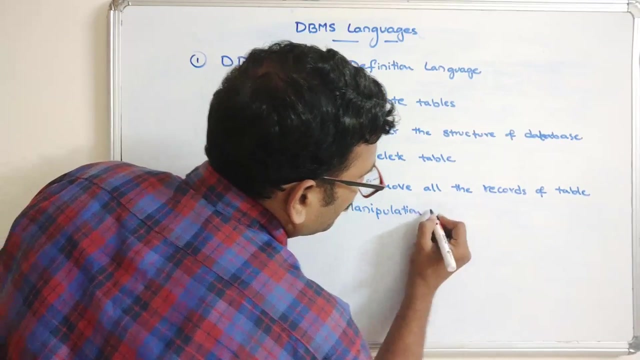 All the records, all the records of database, All the records of the table. okay, so These are the few commands comes under the data definition language. So that's the first language and the second one, Dml. so dml stands for data Manipulation Language, so here: 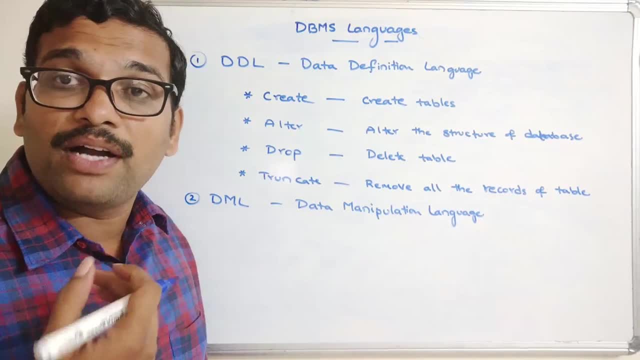 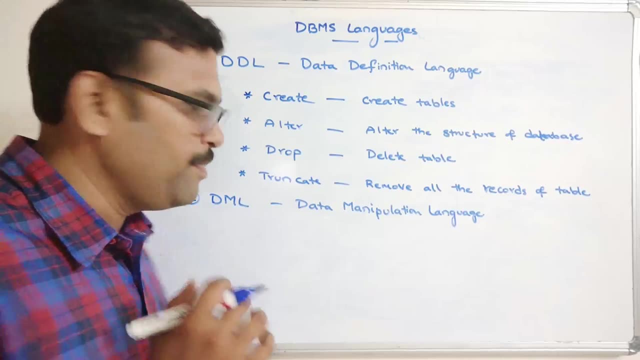 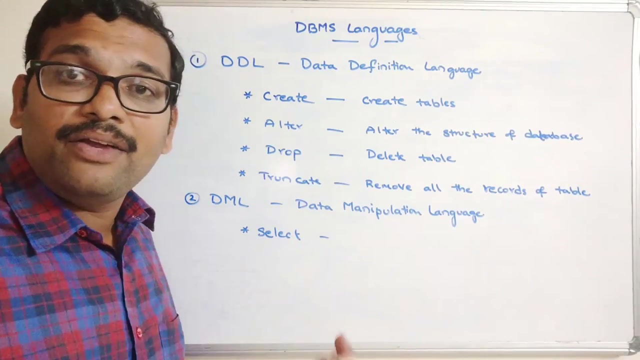 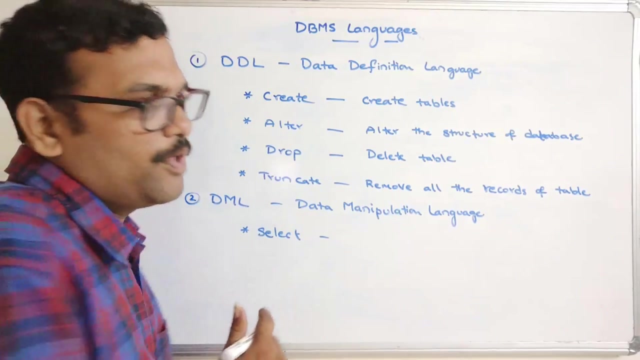 The name itself indicates data manipulations. that means whatever the manipulations We are going to do on the data, that commands will comes under this dml. So first one, select. So select command is used to retrieve the data from the database. That means if you want to get the data, so we have going to use the command called select. Okay so. 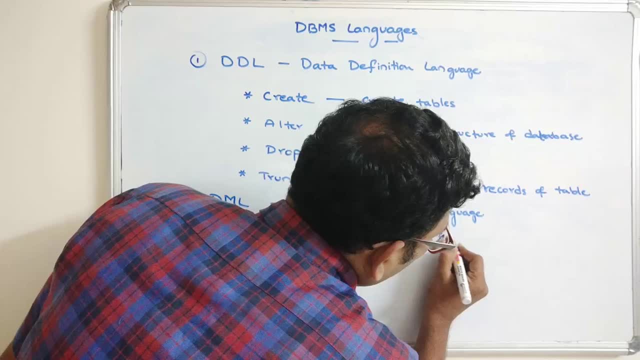 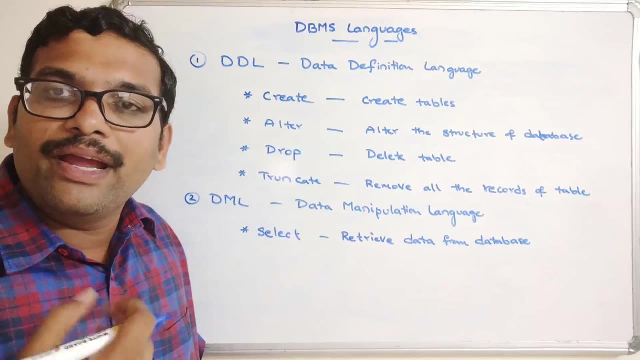 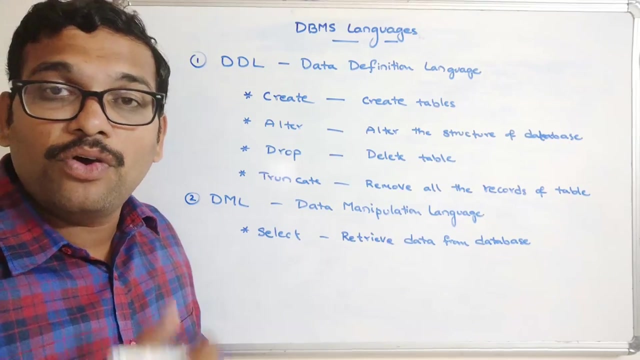 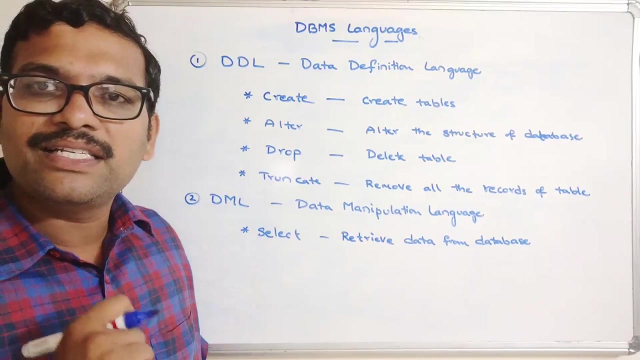 Retrieve data from database. So, For example, I'll share some student table, So I need to get the student details, All the student details who got greater than 90%. So we need to get the selective data from the table student. So for that purpose we are going to use this select command, select command. 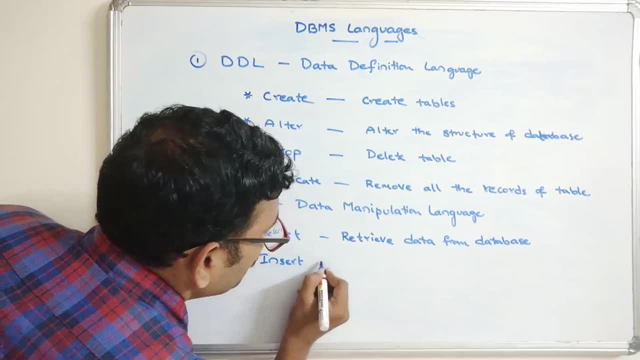 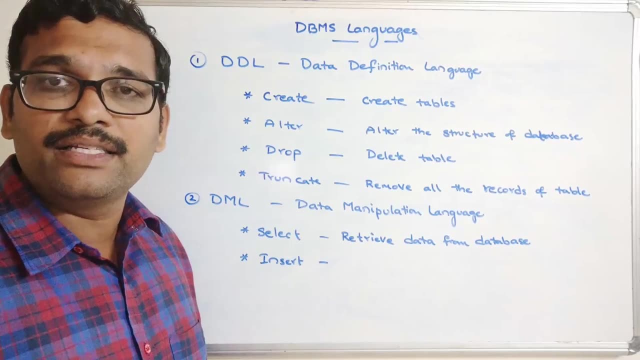 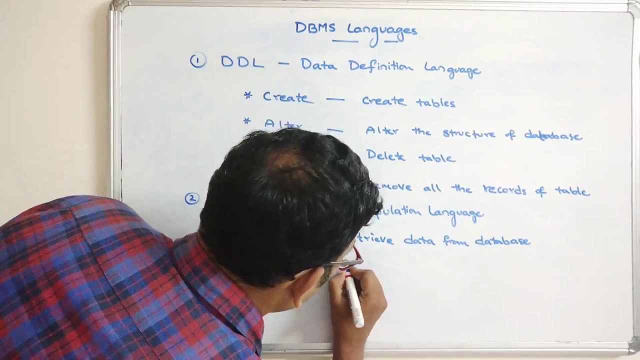 and the next one Insert. so insert command is used to Insert the data into database. So if you want to add a student details, So this insert method will use user to insert the rows of a table cross into a table right. So This is user to insert. 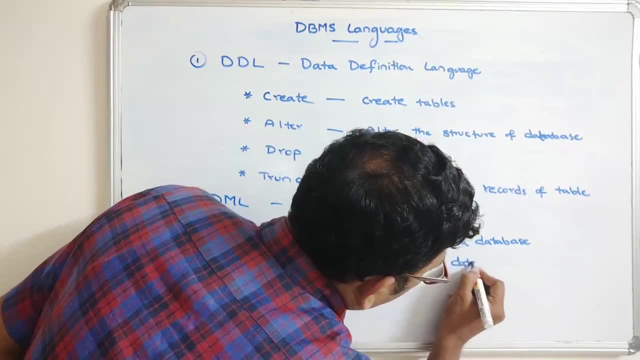 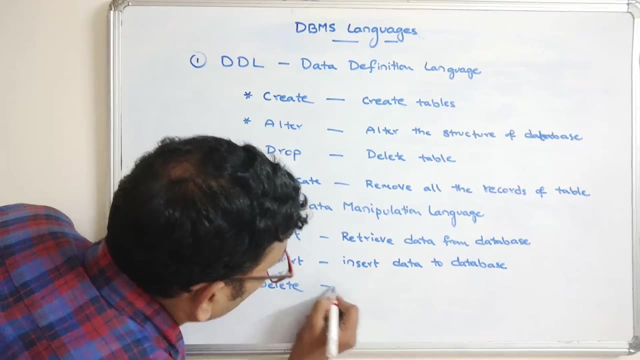 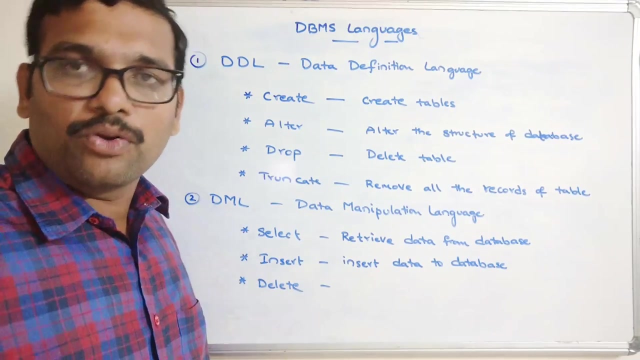 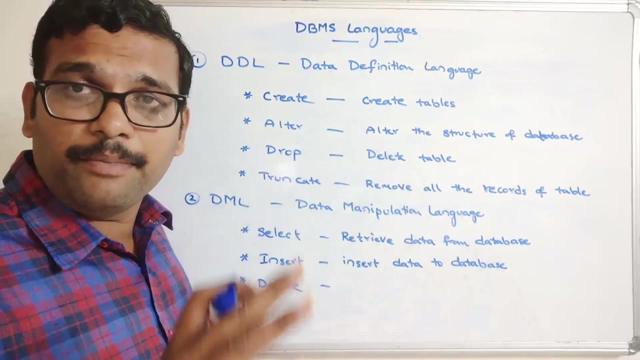 data to the database. So the database and the next one, so quite opposite. that is a delete, and This delete command is used to delete a single row or row Or a multiple rows or all the rows from the table. So it is somewhat different from a time truncate. So truncate will remove all the rows of a database. 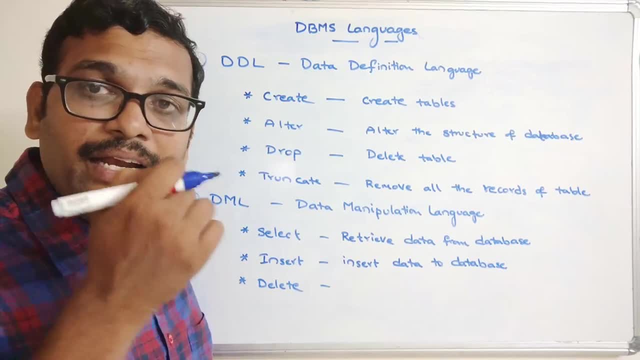 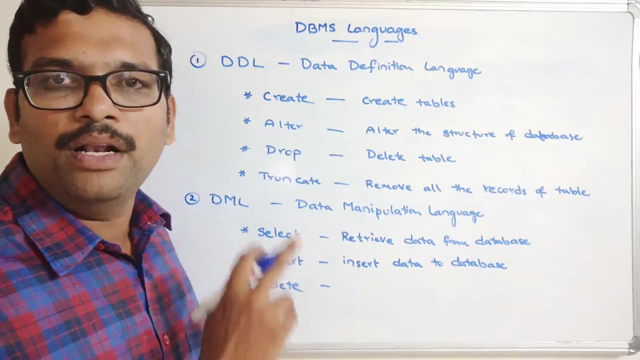 But here delete is used to delete an individual row or a multiple rows or all the rows of a table. right, Based upon the condition we can delete the rows of a table. for that purpose We are going to use this delete command, So it is used to delete. 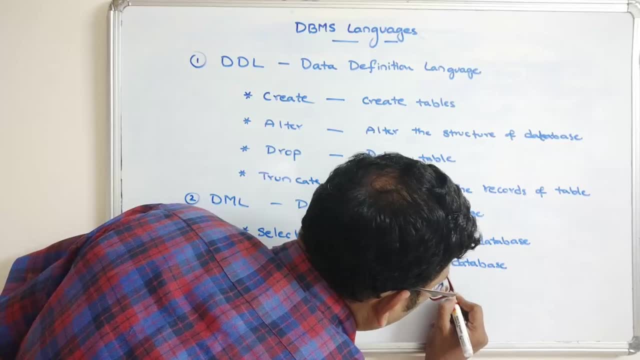 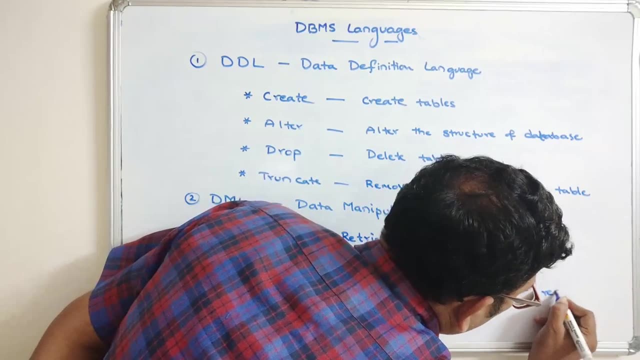 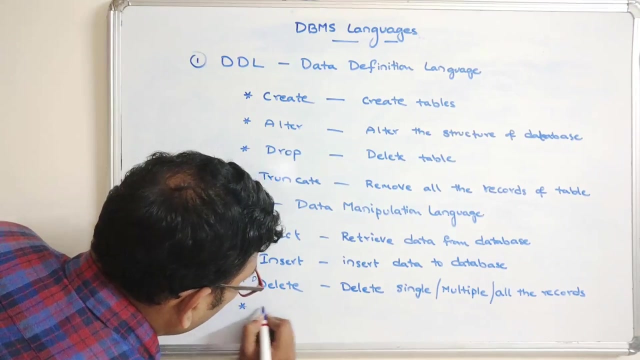 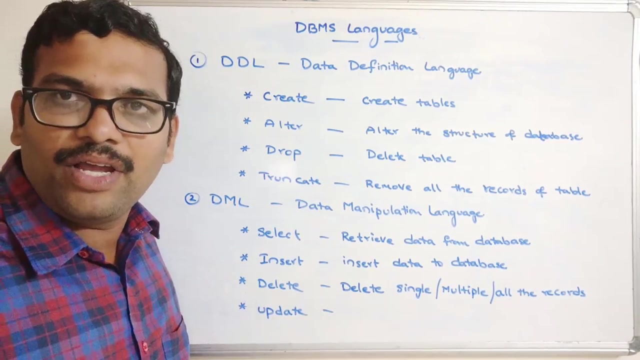 Single or multiple, Or all the records, all the records, Right. so for that we are using delete and the next one update. So this update command is used to update the data. Okay, not the skeleton, not the structure, right? So here we are updating the data, For example, the student. 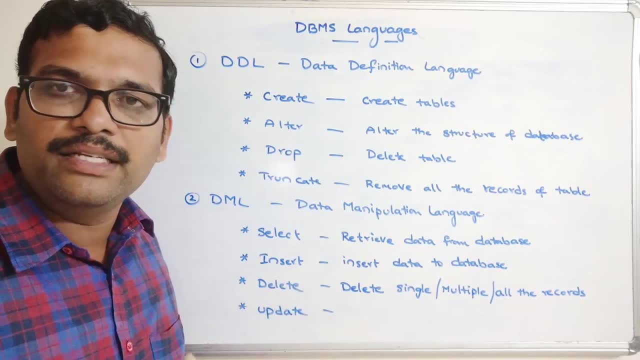 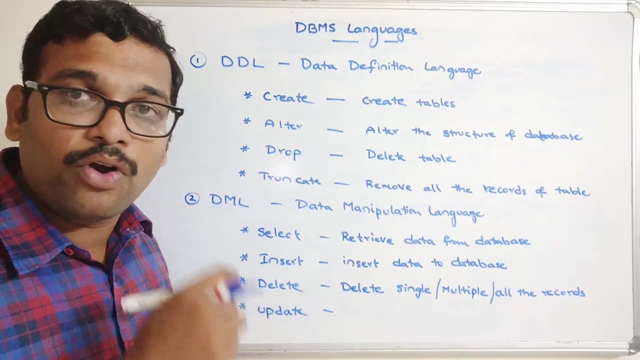 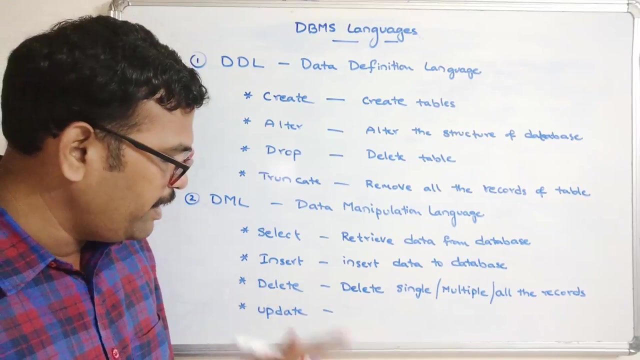 So the student Coming to the student details. So if he got some percentage, Okay. so if we, if we want to update the percentage, okay, now, not the skeleton. So if you want to update the value, okay, update any value of an attribute. that will be done with the help of this update command. 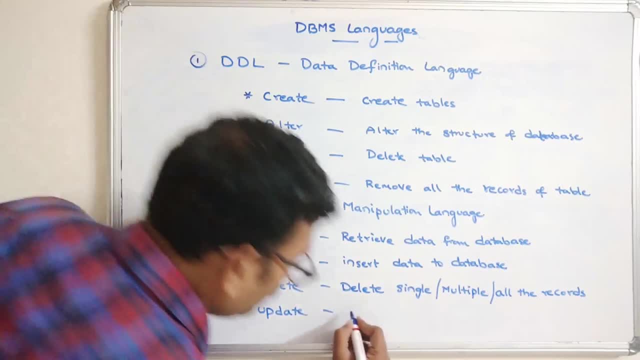 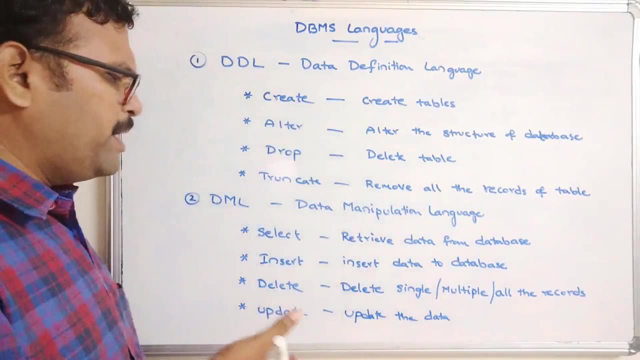 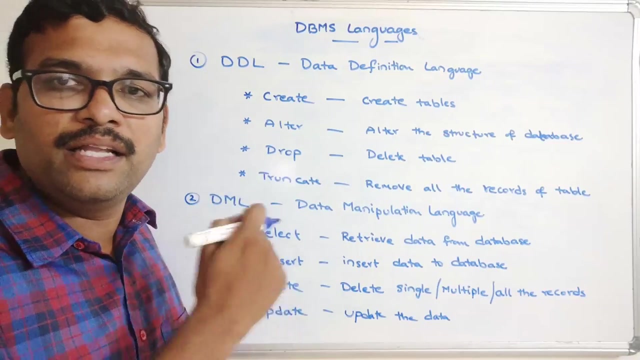 Right: update the data, not the skeleton. So update the data. So these are the very few commands comes under this Data manipulation language. So these are all the commands which are used to Manipulate the data in in the database and this is a DDL, which is a data definition language which will 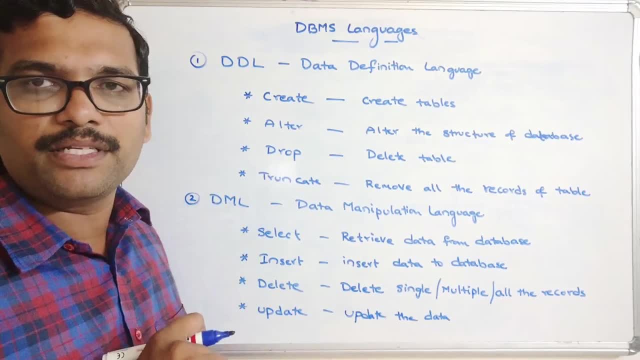 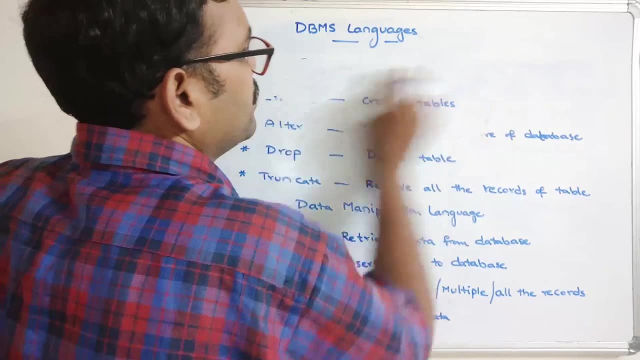 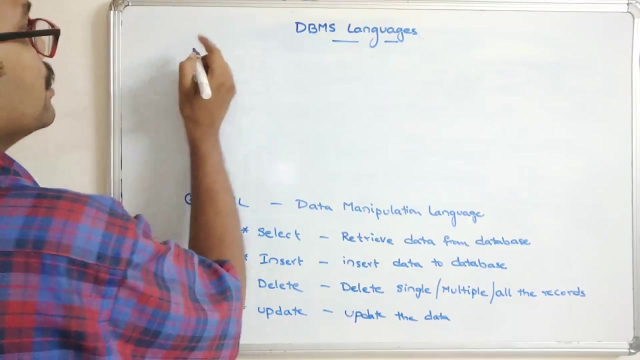 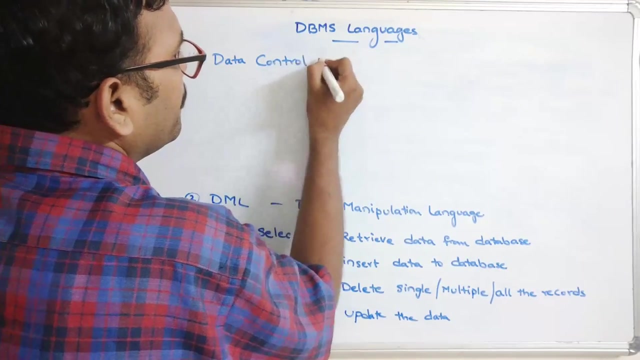 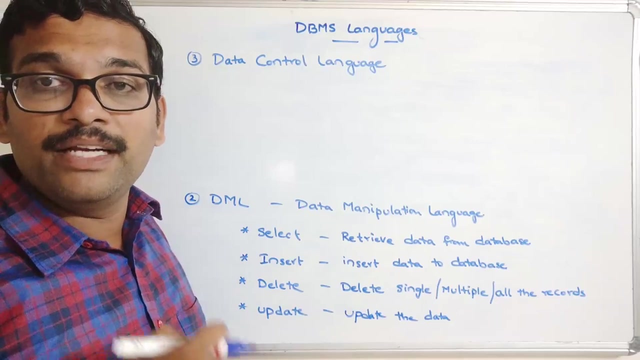 Define the structure of a database. that was a skeleton of a database, Right? So these two are the languages and we will see the third one, that is, Data control language. The third one, data control language, so the control over accessing the data, so the commands which we give the control over accessing the data. so that means we are having a 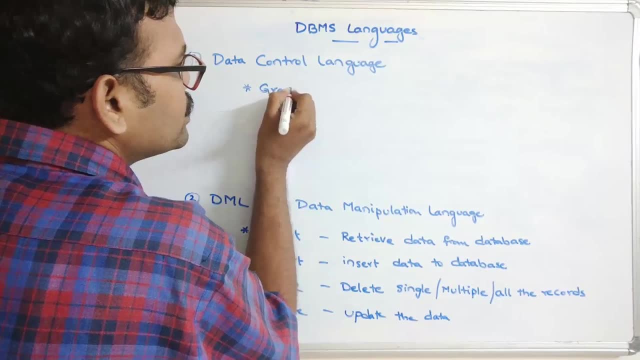 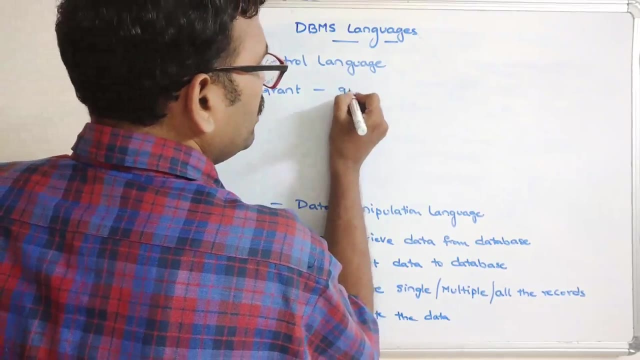 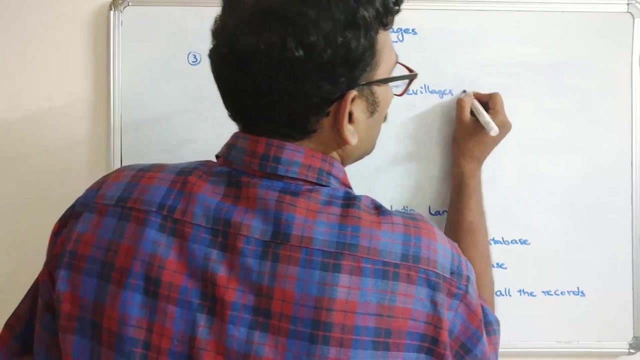 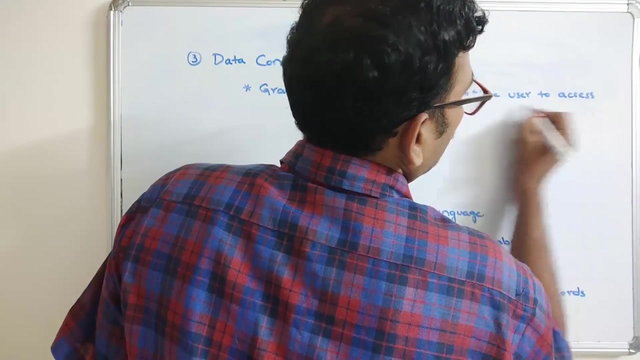 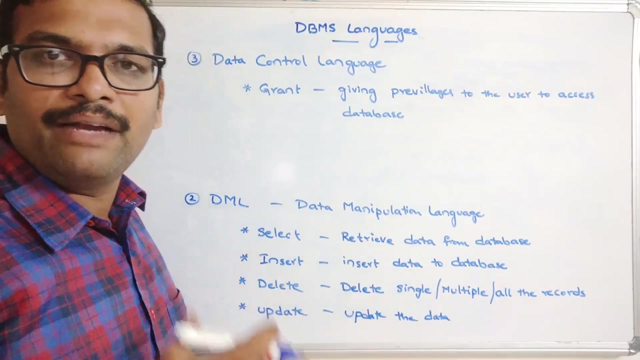 two commands. one is a grant, so this command is used to give the privileges for the user to access the database. okay, so giving privileges or permissions? privileges to the user to access database? okay, giving some permissions, so what type of permissions? so that will be done by this grant command. the next one: 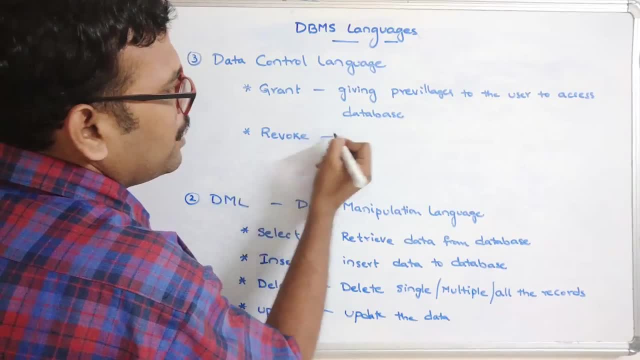 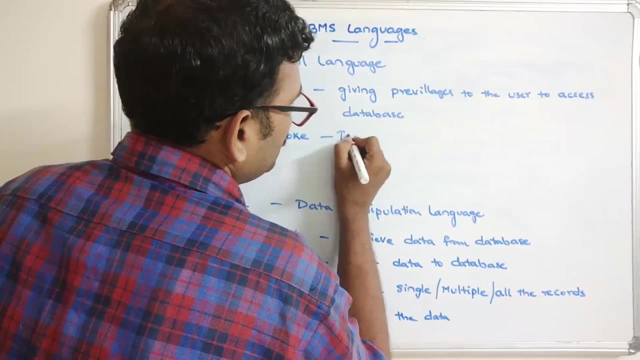 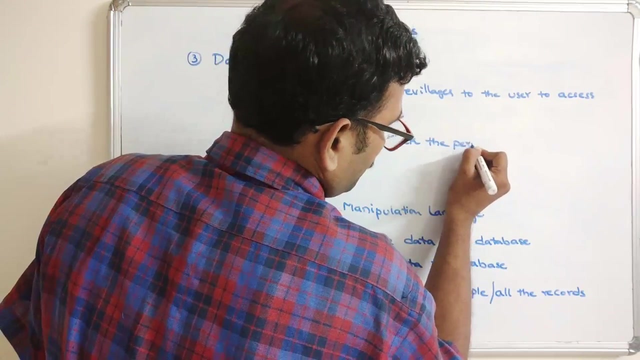 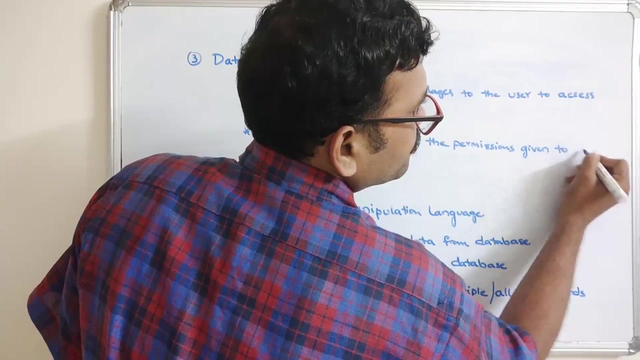 is: revoke. so quite opposite for the grant. so taking all, taking back the permissions from the user. okay, so this is for taking back the permissions or privileges given to user, given to user. taking back the permissions given to given to the user. revoke, so quite opposite for the grant. so taking all. taking back the permissions from the user. okay, so this is for taking back the permissions given to the user. 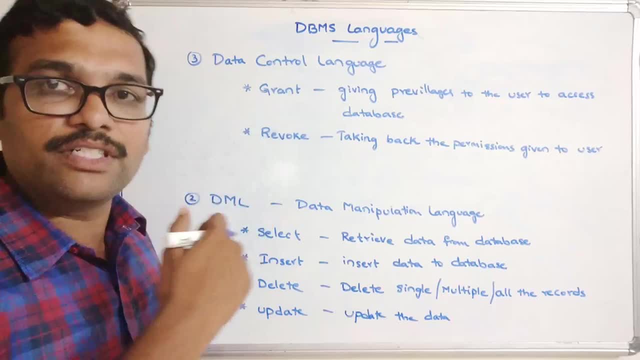 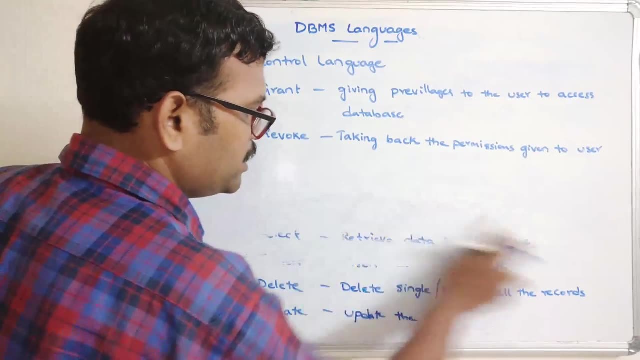 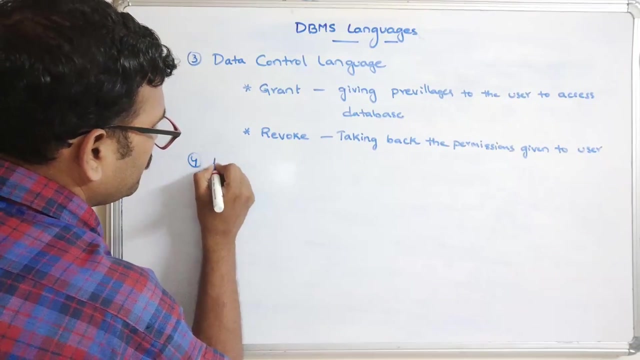 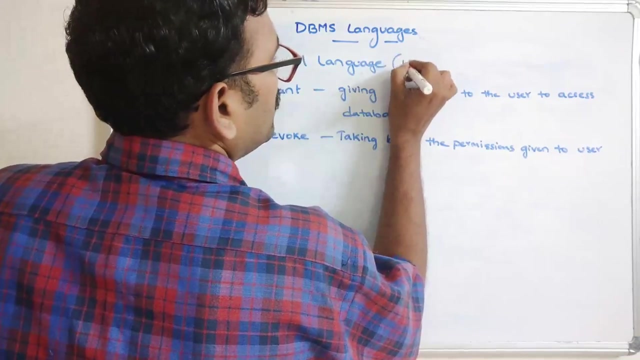 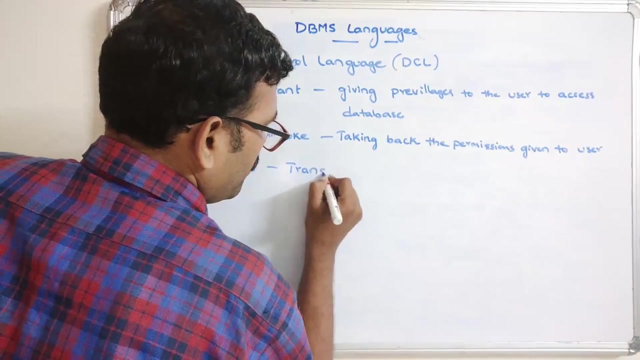 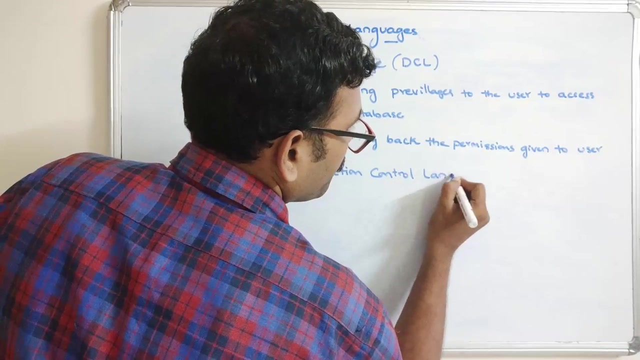 right. so these two comes under this: data control languages, so controlling the accessing of data from the database, right, and the fourth one. the fourth language is a transaction control language, so this is a DCL and this is a DCL, which is transaction control language. so these are the commands comes to. 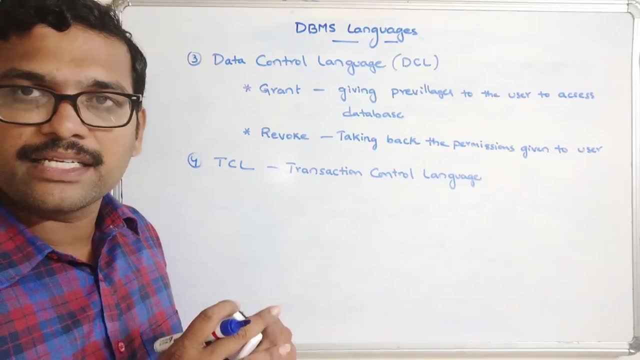 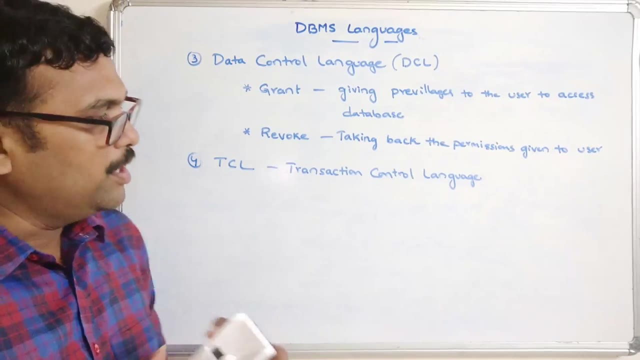 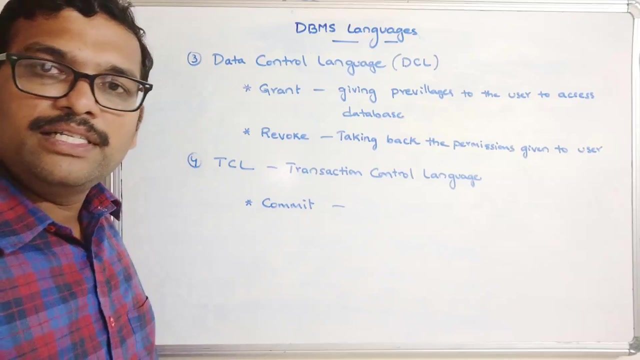 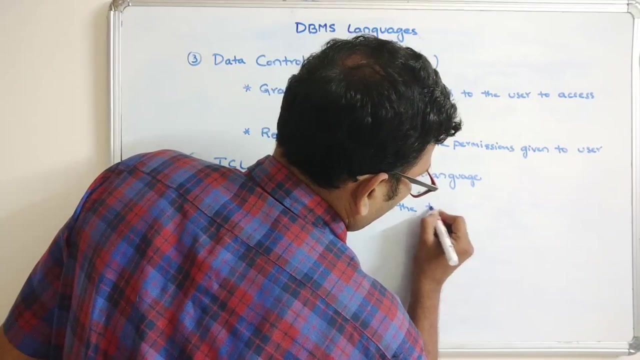 based upon the transactions. okay, coming on the transactions. so whatever the transactions we are doing, so the commands comes under this transaction project. okay, so the fun is commit. so this command is used to save the transaction to the database. okay, save the transaction. save the transaction to the database. 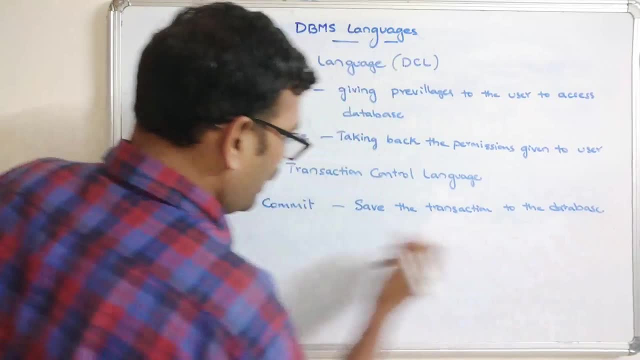 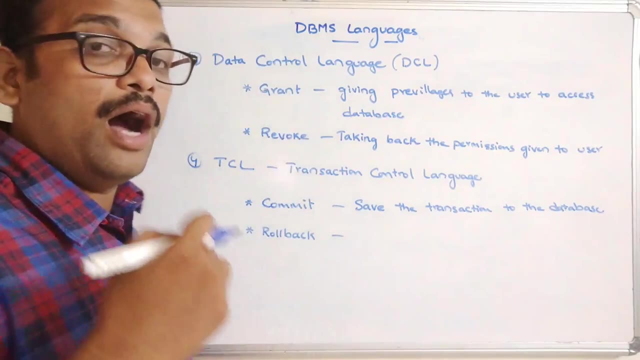 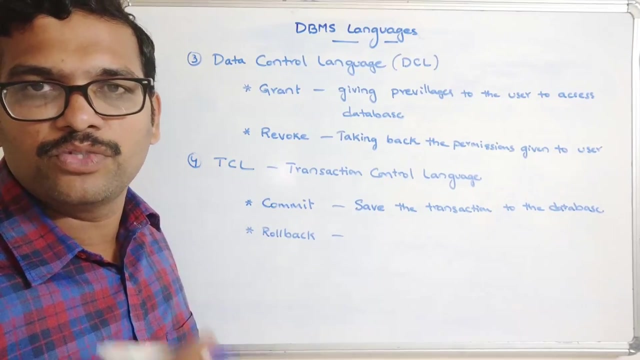 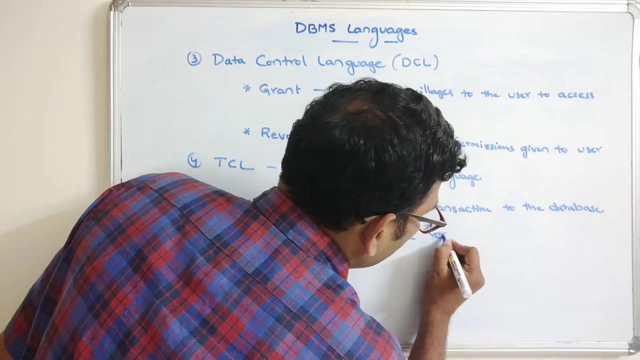 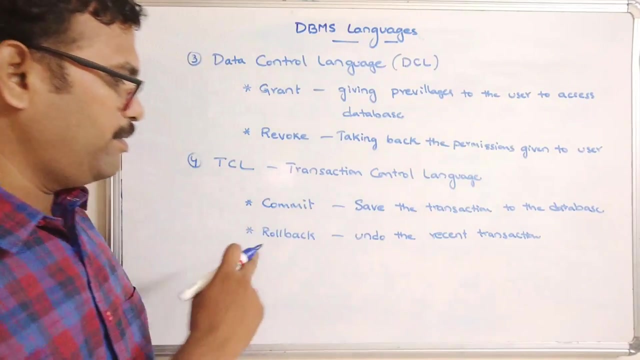 and coming to the next one, that is, rollback. rollback is to undo the transactions which being done in the latest right. that means cancelling the transaction which was done recently, right, so undoing the transaction, undo the transaction, or undo the recent transaction, undo the recent transaction. so that will be done by using this rollback. so these two commands will be work on the 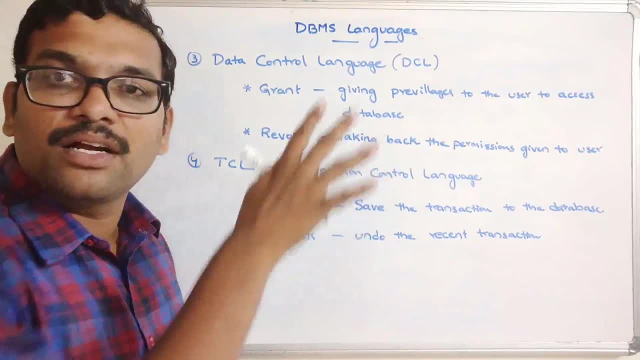 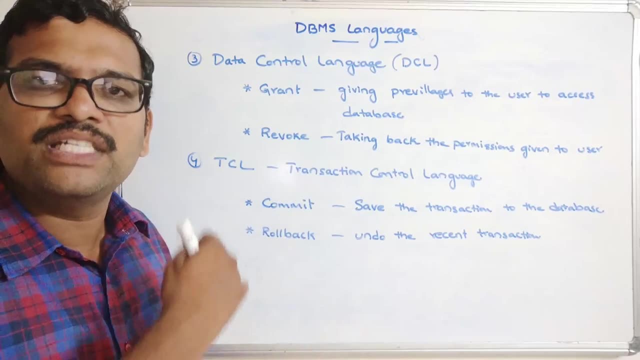 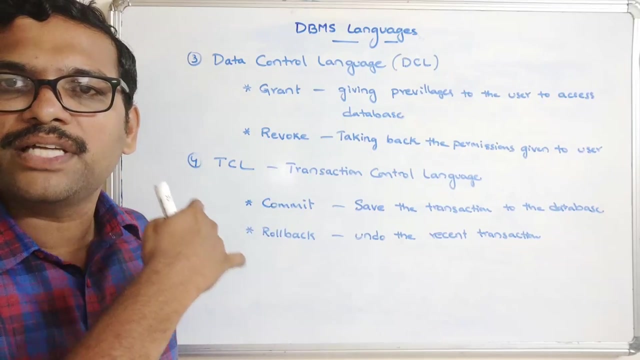 transactions. so these two commands comes under the transaction control language. so we have discussed very few commands, so there are a lot of commands. so these are the very few commands comes under this languages. so data definition language, data manipulation language, data control language and transaction control language. so once we see the summary and we 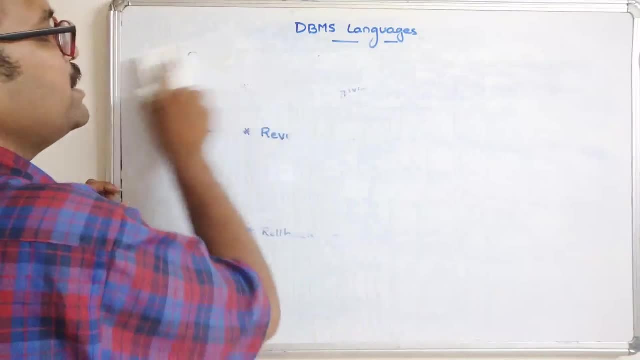 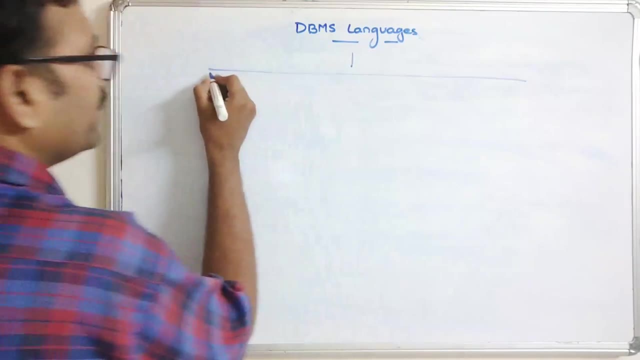 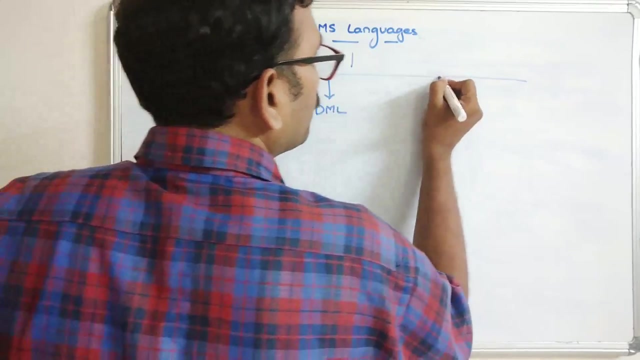 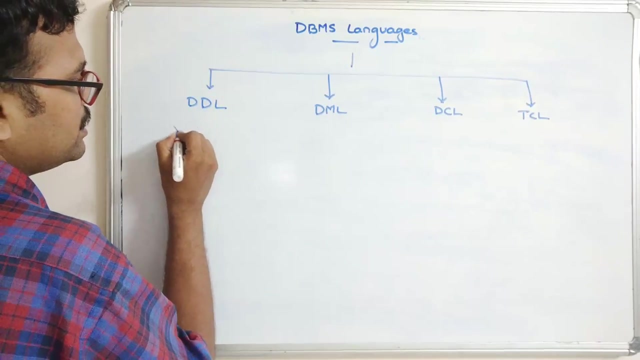 close the session. right, so let me write the commands and languages as a summary. so these languages comes under four categories. so one is ddl, another one is dml, another one is dcl and the last one is pcl. so the commands comes under this ddl are create command. so very few comments there. 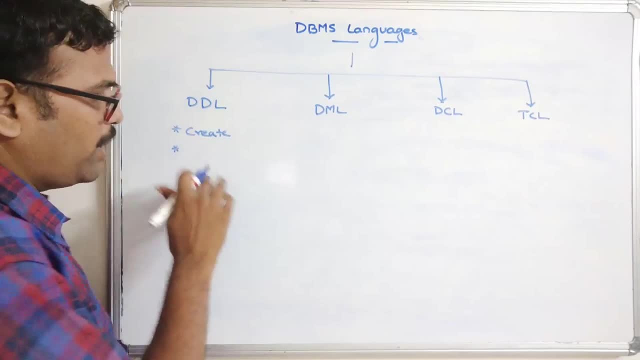 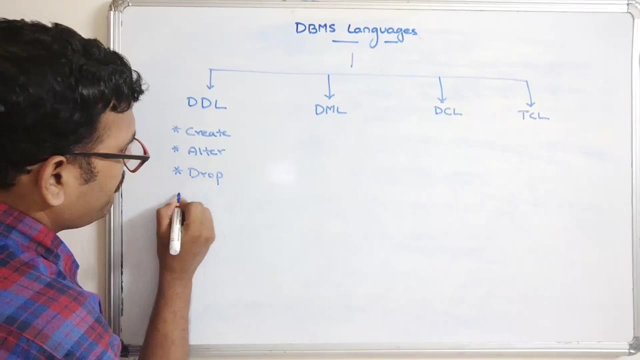 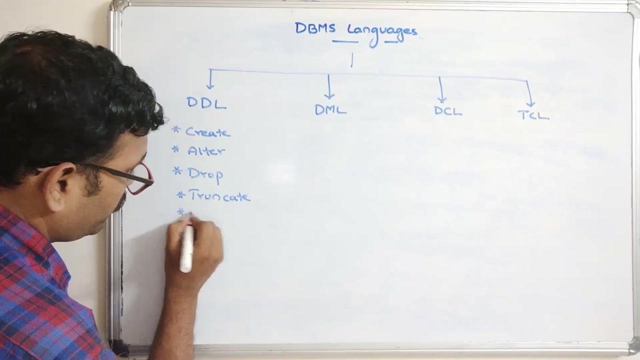 will be lot of comments, but I am writing few comments, so let me just write the last one. only few commands. so alter, drop, truncate, so these are the very few commands. and also rename- okay, in order to rename the table. so we will use this dll, right so?